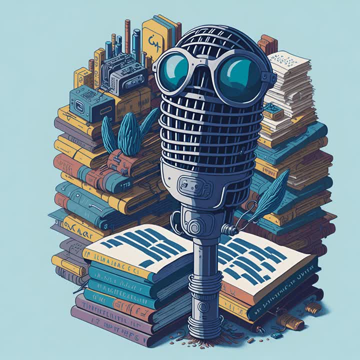 Welcome to Exam English Podcast, where you can practice your English listening skills. Our listening practices follow the style of TOEFL, IELTS, Pearson Test of English and primarily focus on campus-based lectures and conversations. In each episode we explore a different domain of knowledge, from science and engineering to 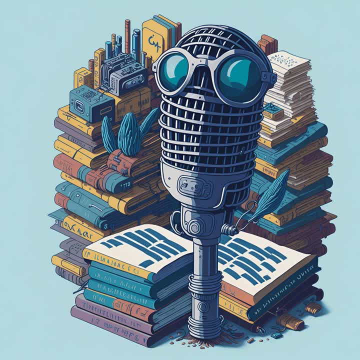 social science. Through our lectures, you'll quickly gain knowledge in a variety of subjects. Today, we are going to talk about biomedical engineering and medical devices from the perspective of biomedical science. Good morning everyone. Biomedical engineering and medical devices is an 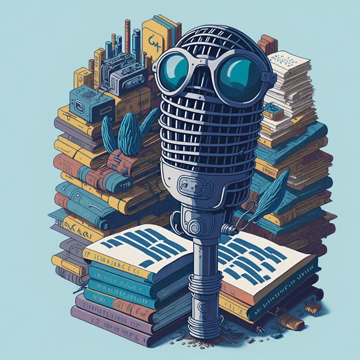 interesting and complex subject area. In simple terms, biomedical engineering and medical devices are things that are used in and around us to diagnose, monitor and treat diseases. Oh, let's take a look at some of the historical aspects of biomedical engineering and medical devices. Well, traditionally, engineering began in the 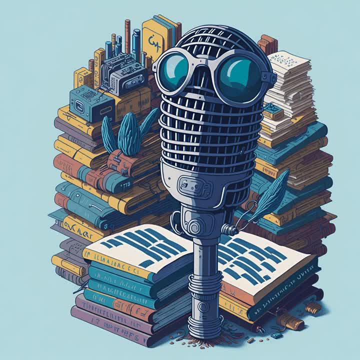 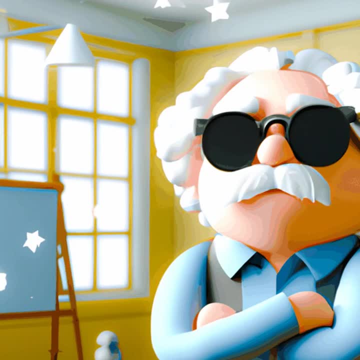 18th century, which is why we see so many historically significant achievements related to biology and medicine, For example, advances in surgical instruments from the 19th century or ones we still use today, Such as the stethoscope 口毟' Right. There are advantages and disadvantages of using biomedical engineering. 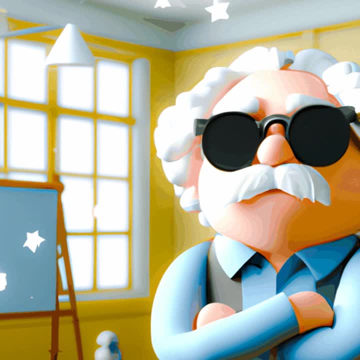 and medical devices. The advantages are that it has allowed for precision, diagnosis, precise treatments and innovations in the laboratory world. It increases our understanding of the human body and its workings. The disadvantages, however, can be seen when it comes to cost, complexity and medical errors. 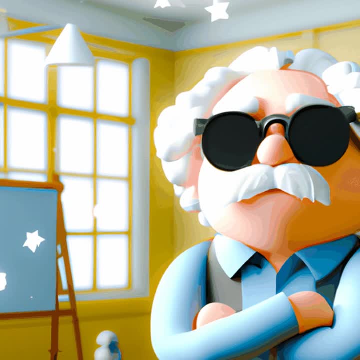 Let's look at some real-world examples of biomedical engineering and medical devices. We can take a look at things like prosthetics, pacemakers, hearing aids, heart valves and artificial hearts. These devices are all designed to mimic the functionality of the human body. 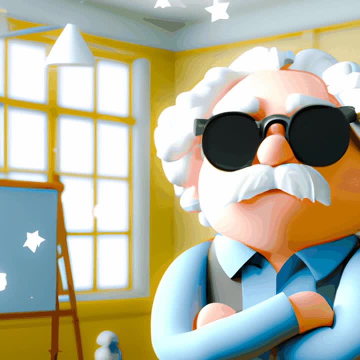 to help improve the lives of those living with medical conditions. So, looking to the future, we can anticipate advances in areas such as artificial intelligence, nanomedicine and robotics, which could help revolutionize the medical field. Furthermore, there are other techniques, such as gene editing. 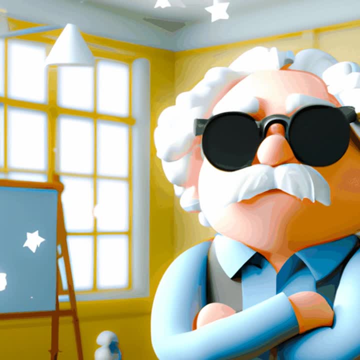 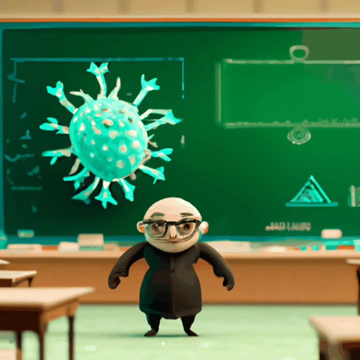 3D printing and tissue engineering, which can also be combined with biomedical engineering and medical devices to further improve treatment and diagnosis. Here is the summary of the lecture regarding biomedical engineering and medical devices from the perspective of biomedical science. To summarize, biomedical engineering and medical devices can be seen in a number of ways. 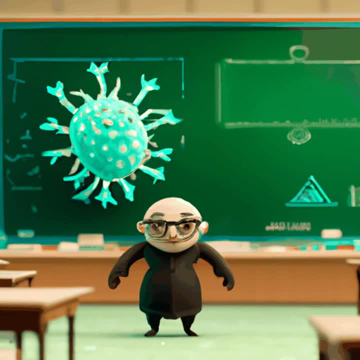 from traditionally looking at surgical instruments of the 18th century to current prosthetics, pacemakers and other medical devices we use today. we use today. There are, of course, advantages and disadvantages. However, the future looks bright with the potential of advances such as artificial intelligence and nanomedicine. 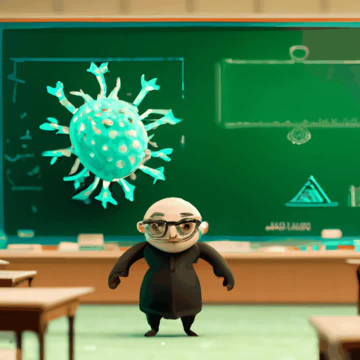 to help revolutionize the medical field. Now the lecture is going to repeat and speaking rate goes back to normal. Good morning everyone. Biomedical engineering and medical devices is an interesting and complex subject area. In simple terms, biomedical engineering and medical devices are things: 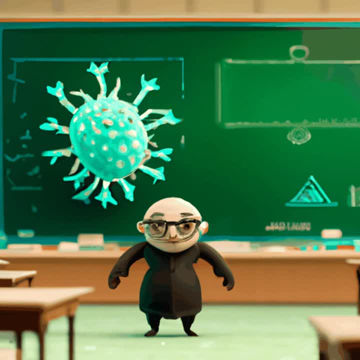 that are used in and around us to diagnose, monitor and treat diseases. Oh, let's take a look at some of the historical aspects of biomedical engineering and medical devices. Well, traditionally, engineering began in the 18th century, Which is why we see so many historically significant achievements related to biology. 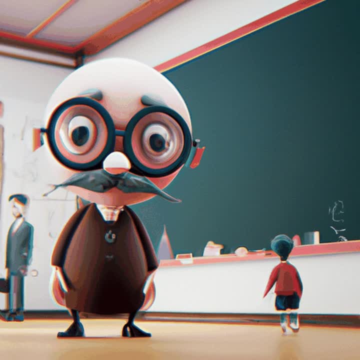 and medicine, For example, advances in surgical instruments from the 19th century or ones we still use today, such as the stethoscope. Hmm, of course, there are advantages and disadvantages to using biomedical engineering and medical devices. The advantages are that it has allowed for precision, diagnosis, precise treatments and 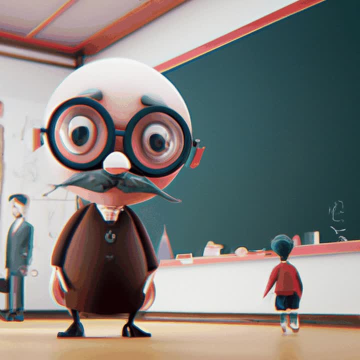 innovations in the laboratory world. It increases our understanding of the human body and its workings. The disadvantages, however, can be seen when it comes to cost, complexity and medical errors. Hmm, let's look at some real-world examples of biomedical engineering and medical devices. 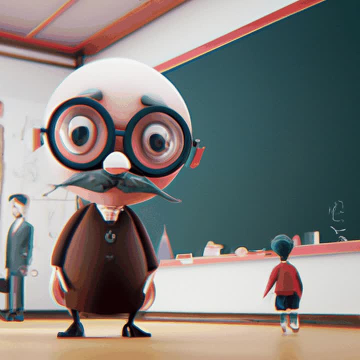 We can take a look at things like prosthetics, pacemakers, hearing aids, heart valves and artificial hearts. These devices are all designed to mimic the functionality of the human body to help improve the lives of those living with medical conditions. So, looking to the future, we can anticipate advances in areas such as artificial intelligence. 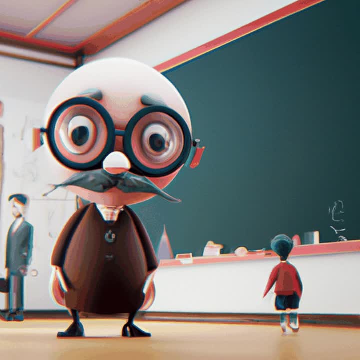 nanomedicine and robotics, which could help revolutionize the medical field. Furthermore, there are other techniques, such as gene editing, 3D printing and tissue engineering, which can also be combined with biomedical engineering and medical devices to further improve treatment and diagnosis. 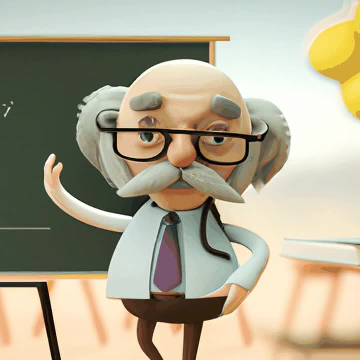 So let's look at some of the advantages and disadvantages of biomedical engineering and medical devices Sound hoof. I'll leave it up to you to discuss where the leading indicators are consensual. Following the lecture, a student approached the lecturer in their office with questions about 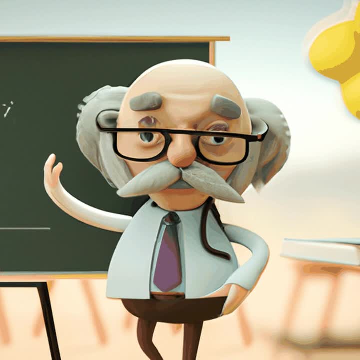 the definition and concept of biomedical engineering and medical devices. Hey Dr Frizl, I'm really interested about biomedical engineering and medical devices. Can you tell me more about them? is the application of engineering principles to solve medical problems. Medical devices are tools used to diagnose and treat illness and medical conditions. 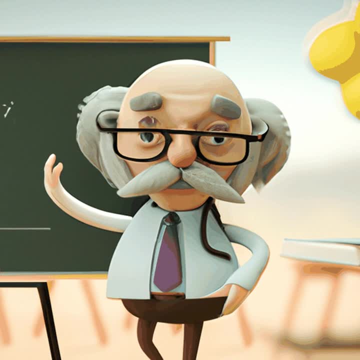 So together they allow us to improve healthcare. Oh wow, that's really cool. So can you give me an example of a medical device? Sure, For example, one type of medical device is a pacemaker. Pacemakers are used to regulate abnormal heart rhythms so that the heart can beat at a steady and regular pace. 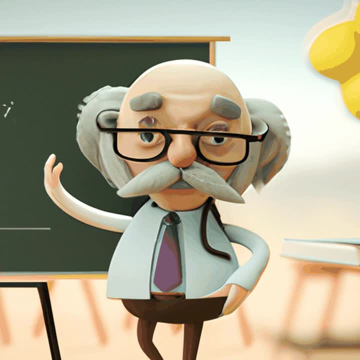 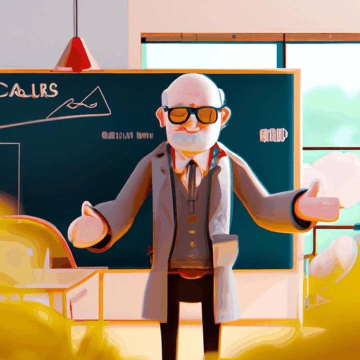 Like they contain a small generator which sends electrical signals to the heart muscle, So they help to maintain a normal heart rhythm. Now the discussion is going to repeat and speaking rate goes back to normal. Thank you for watching. Hey, Dr Frizzle, I'm really interested about biomedical engineering and medical devices.